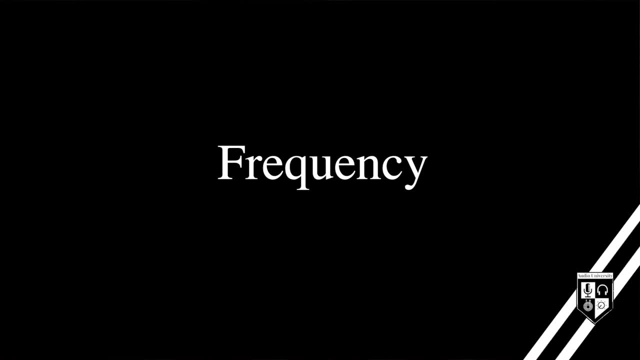 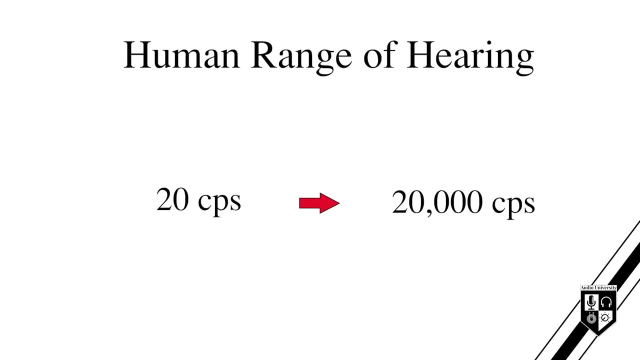 second Frequency describes how many of these cycles are completed per second. Humans are capable of hearing sounds in the range of 20 cycles per second to 20,000 cycles per second. Frequency corresponds to musical pitch, although musical pitch is affected by other factors, as 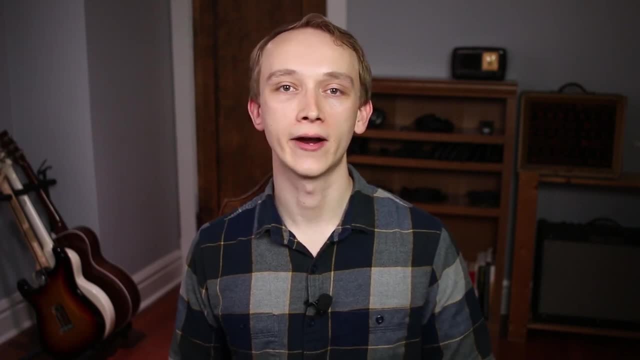 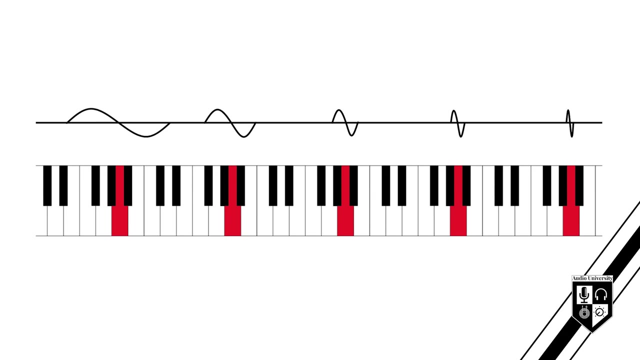 well, Generally speaking, the higher the frequency, the higher the pitch. For example, if you double the frequency of a sound, the pitch of the sound will rise by one octave. If you cut the frequency in half, the pitch of the sound will decrease by one octave. 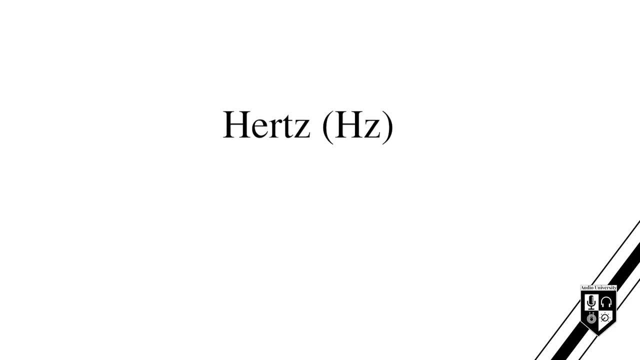 Frequency is measured in hertz, abbreviated HZ. One cycle per second. per second is 1 kilohertz. As I stated before, humans are capable of hearing sounds within the range of 20 cycles per second and 20,000 cycles per second. In other words, they're capable of. 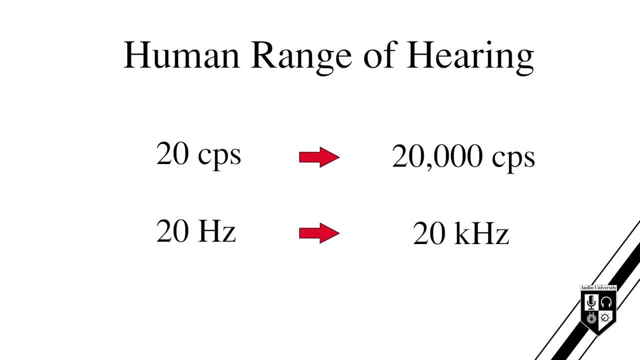 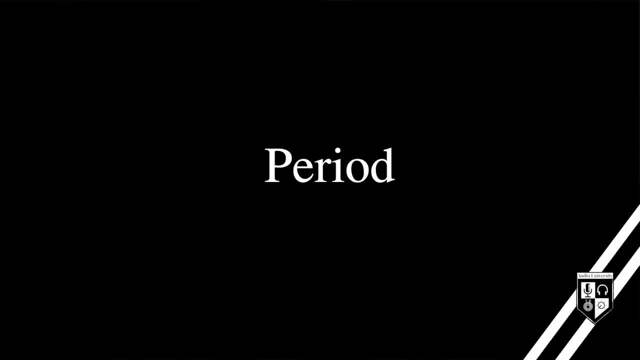 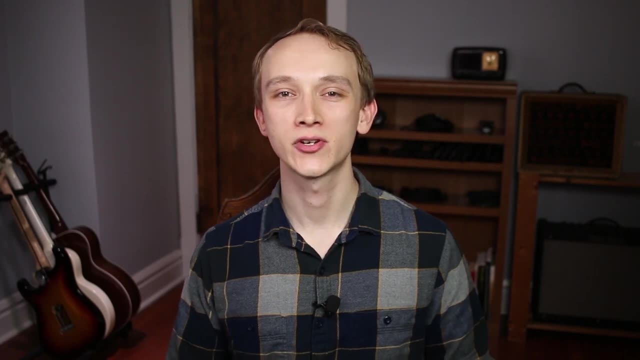 hearing sounds in the range of 20 hertz to 20 kilohertz. Whereas frequency describes how many cycles are completed per second, the period of a wave describes how many seconds it takes to complete one cycle. Period is therefore a measurement of time and is measured in seconds. 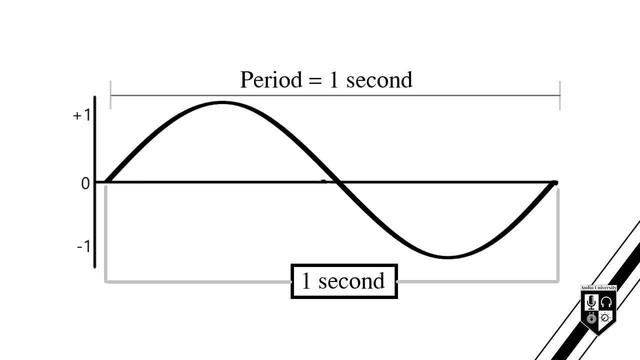 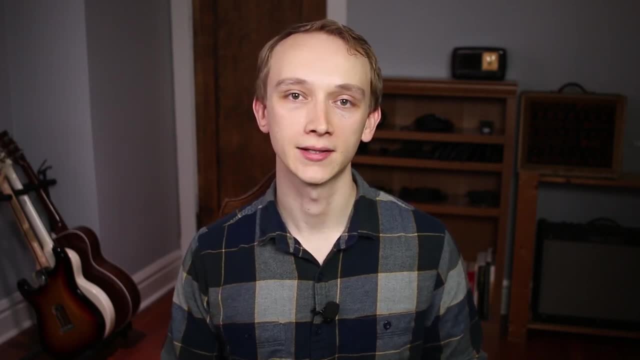 or usually milliseconds. A sound wave with a frequency of one hertz has a period of one second. A sound wave with a frequency of two hertz has a period of half of a second. As you get up into the audible range above 20 hertz, milliseconds become a lot more useful than seconds. Wavelength: 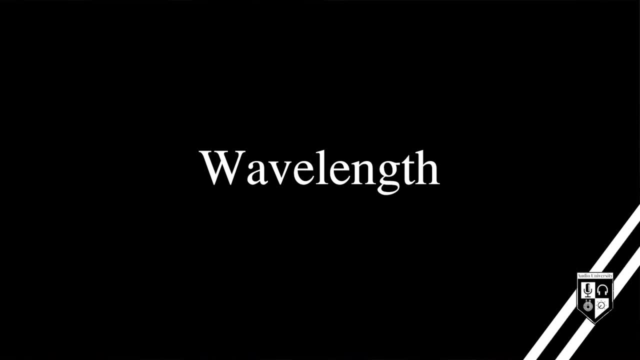 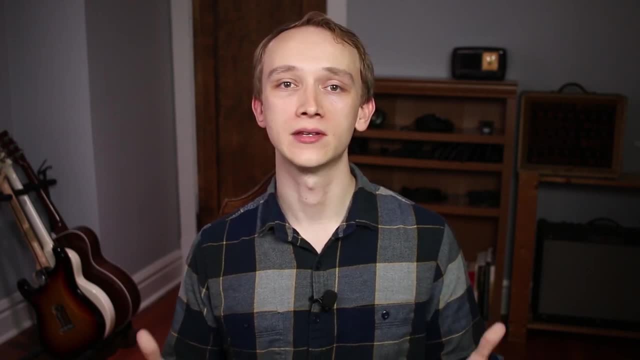 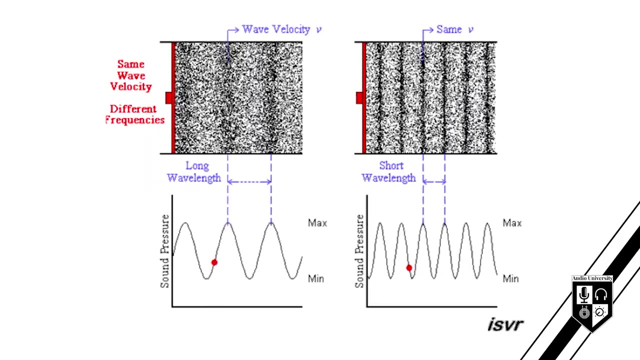 and period are very often confused, but they're different. Period is a measurement of time. wavelength is a measurement of distance. Wavelength describes the physical distance it takes a sound wave to complete one cycle. Here's an animation created by ISVR. 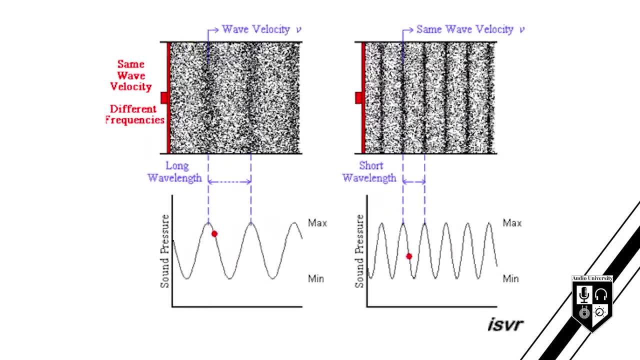 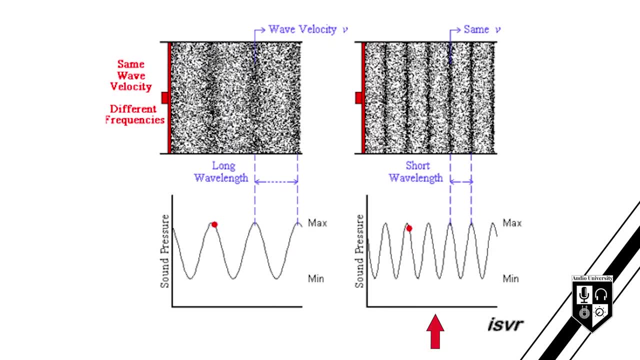 I've linked to it in the description of this video. It's really helpful in showing the relationship between frequency and wavelength. Lower frequencies have longer wavelengths, whereas higher frequencies have shorter wavelengths. To calculate the wavelength of a given frequency, use this formula. 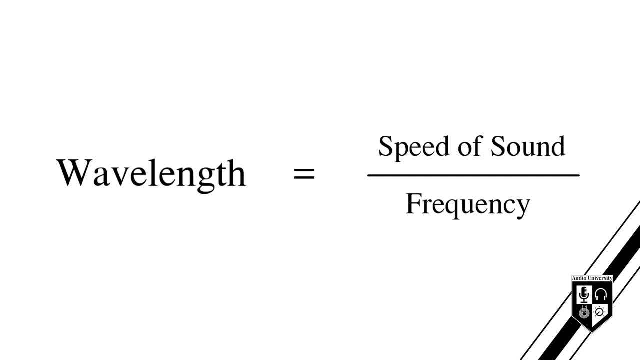 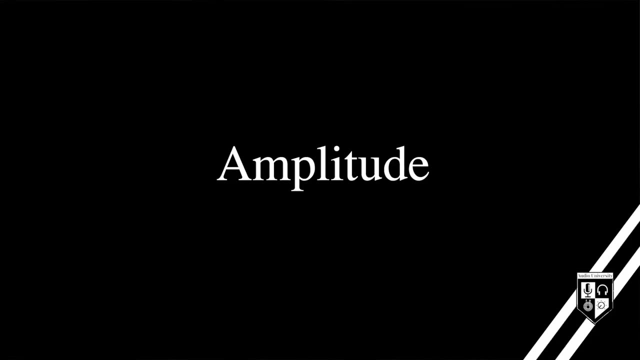 Speed of Sound divided by frequency. Although differences in temperature and humidity can have an effect on the speed of sound, using the standard 1130 feet per second as the speed of sound in this formula will give you a very close to accurate result. Amplitude describes the extent of the pressure changes. Higher amplitude.